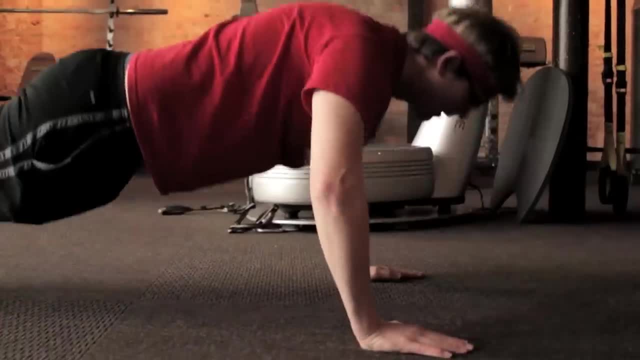 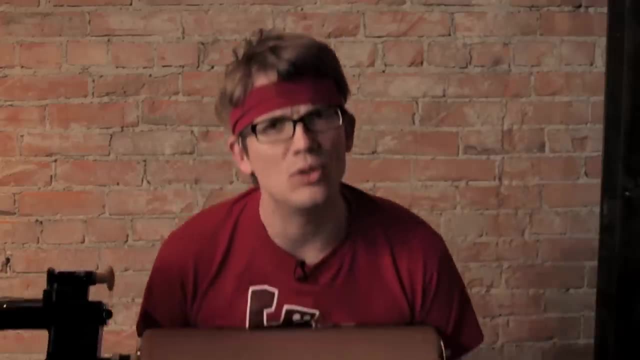 Ugh, You see what happened there. My arms moved, my shoulders moved, my back and stomach muscles moved, my heart pumped blood to all those different places. It's pretty neat, huh? Well, it turns out that how we make and use energy is a lot like sports or other kinds of exercise. 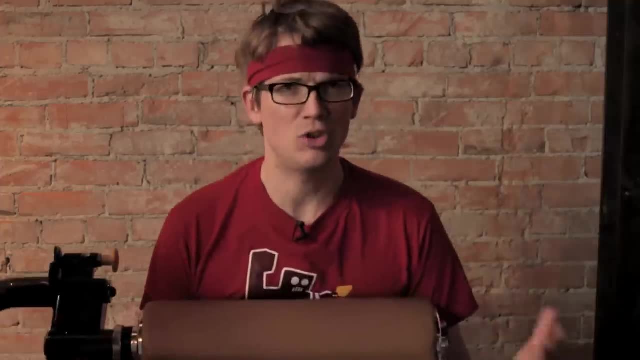 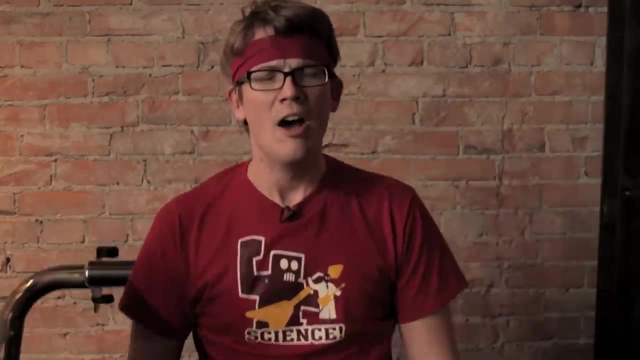 It can be hard work and a little bit complicated, but if you do it right it comes with some tremendous payoffs. But unlike hitting a ball with a stick, it's so marvelously complicated and awesome that we're still unraveling the mysteries of how it all works. 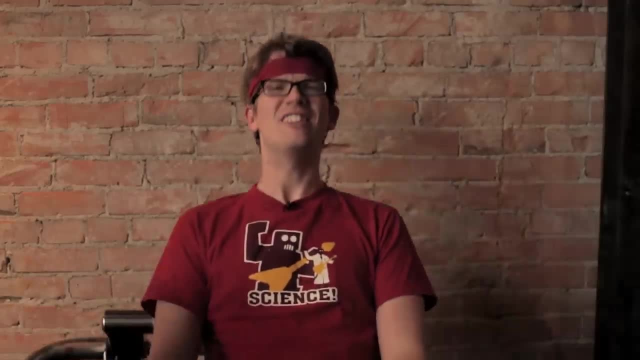 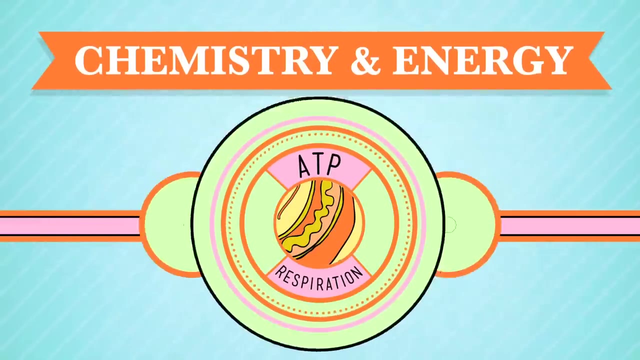 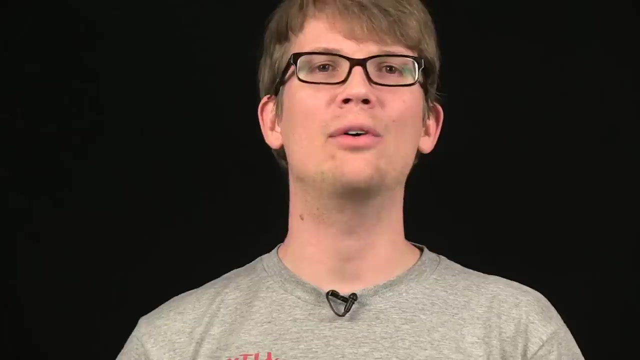 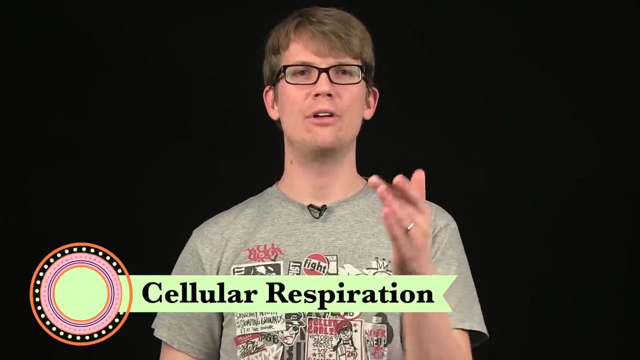 And it all starts with a marvelous molecule that is one of your best friends, ATP. Today, I'm talking about the energy and the process. ourselves And other animals do the same thing. Other animal cells go through to provide themselves with power. Cellular respiration is how we derive energy from the food that we eat, specifically from glucose, since most of what we eat ends up as glucose. 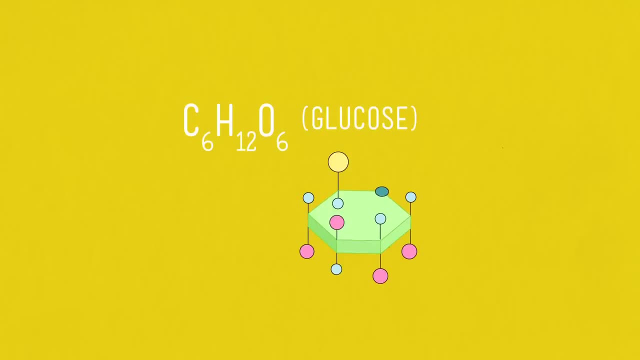 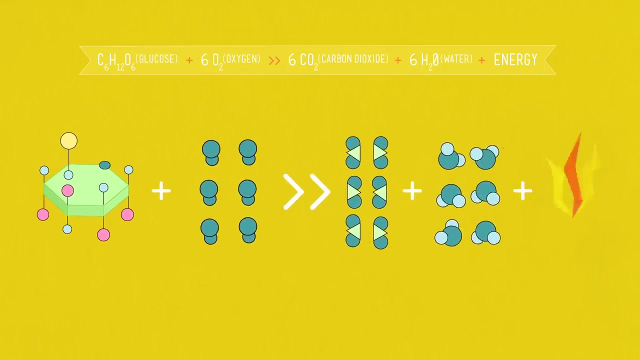 Here's the chemical formula for one molecule of glucose. In order to turn this glucose into energy, we're going to need to add some oxygen, six molecules of it, to be exact. Through cellular respiration, we're going to turn that glucose and oxygen into six molecules of CO2, six molecules of water and some energy that we can use. 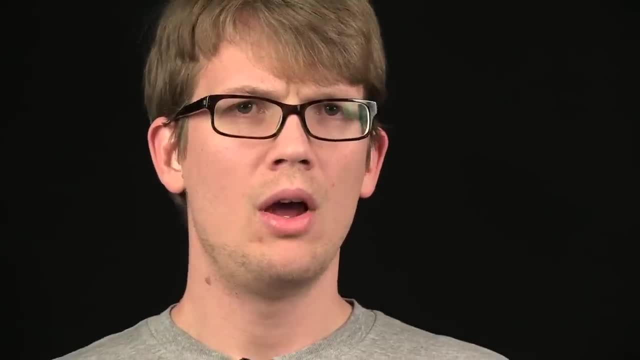 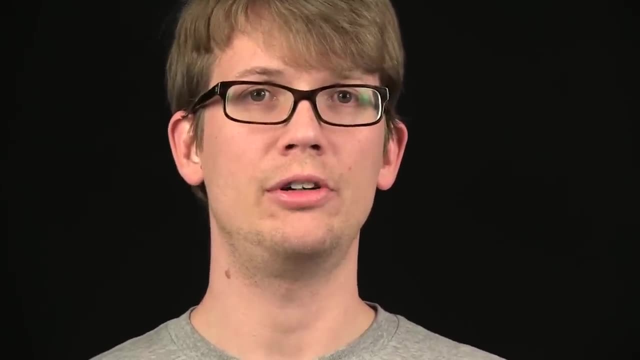 for doing all of our push-ups. So that's all well and good, but here's the thing: We can't just use that energy to run a marathon or something. First our bodies have to turn that energy into a really specific form of stored energy called ATP or adenosine triphosphate. 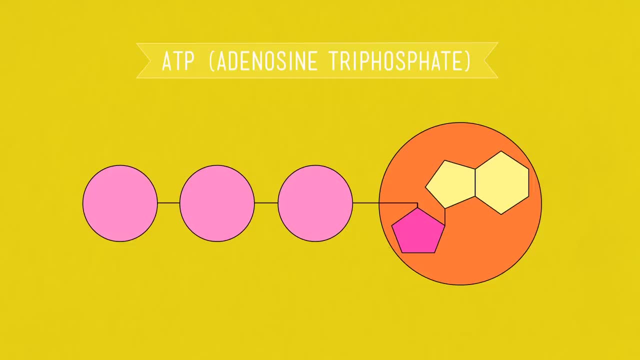 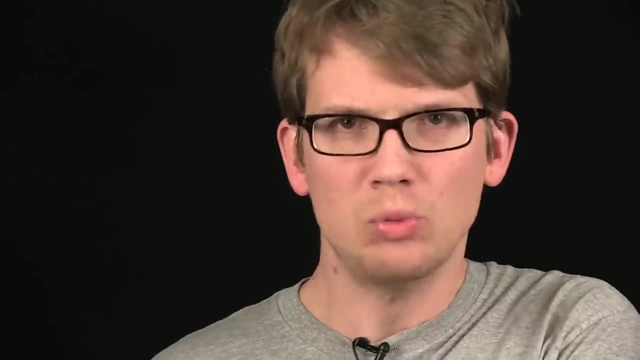 You've heard me talk about this before. People often refer to ATP as the currency of biological energy. Think of it as an American dollar. It's what you need to do business in the US. You can't just walk into a Best Buy with a handful of Chinese yen or 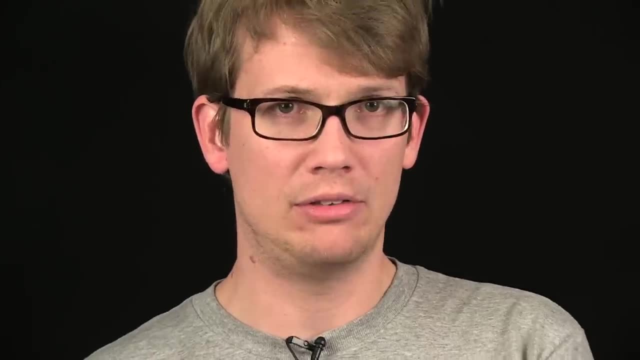 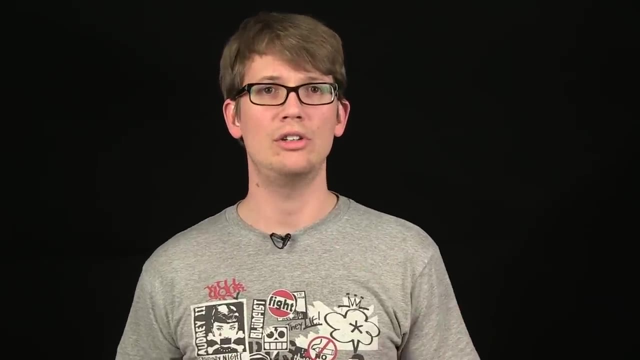 Indian rupees and expect to be able to buy anything with them, even though they're technically our money. Same goes with energy. In order to be able to use it, our cells need energy to be transferred into adenosine triphosphate to be able to grow move. 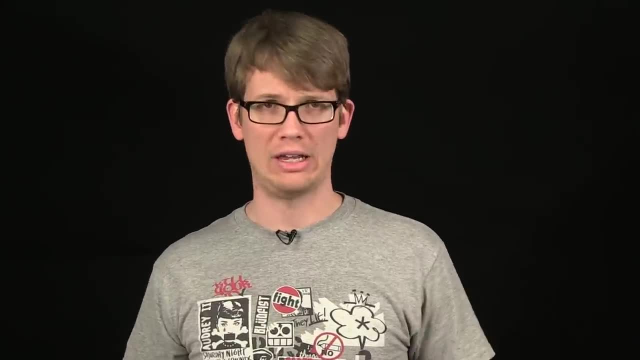 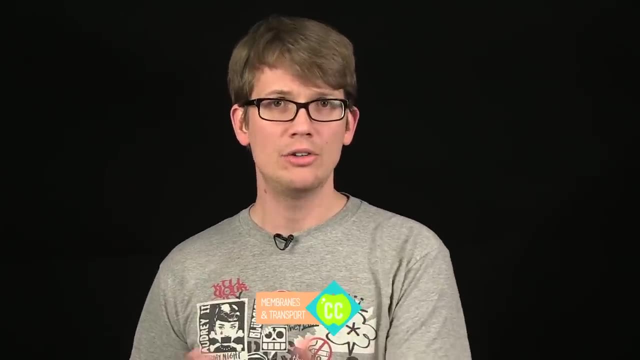 create electrical impulses in our nerves and brains- everything. A while back, for instance, we talked about how cells use ATP to transport some kinds of materials in and out of its membranes. To jog your memory about that, you can watch that episode right here. 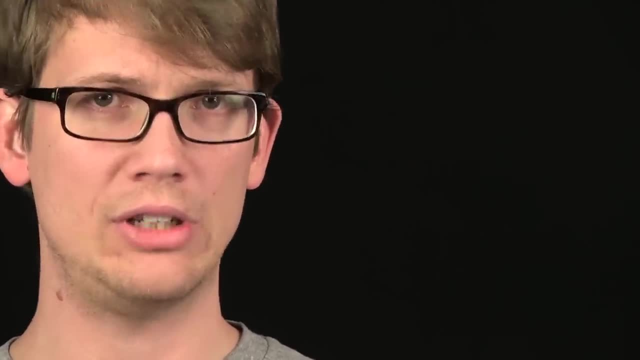 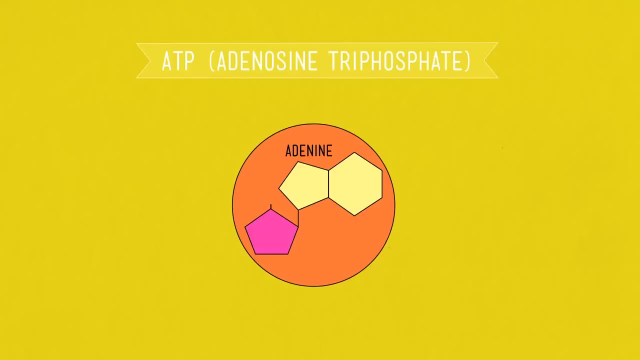 Now, before we see how ATP is actually put together, let's look at how cells can cash in on the energy that's stashed in there. Well, adenosine triphosphate is made up of a nitrogenous base called adenine, with a sugar called ribose and three phosphate groups attached to it. 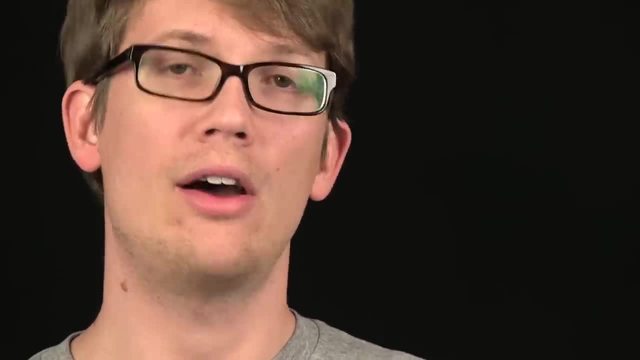 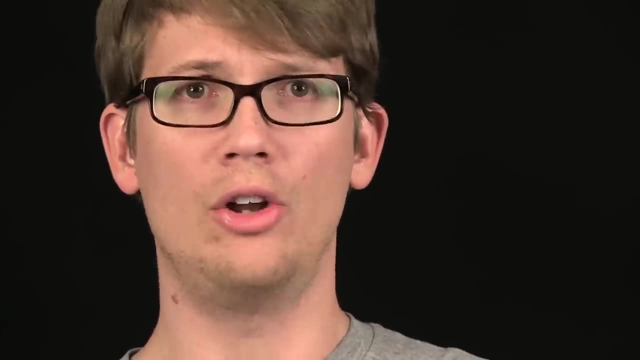 Now, one thing you need to know about these three phosphate groups is that they are super uncomfortable sitting together in a row like that, like three kids on a bus who hate each other, all sharing the same seat. So because the phosphate groups are such terrible company for each other, 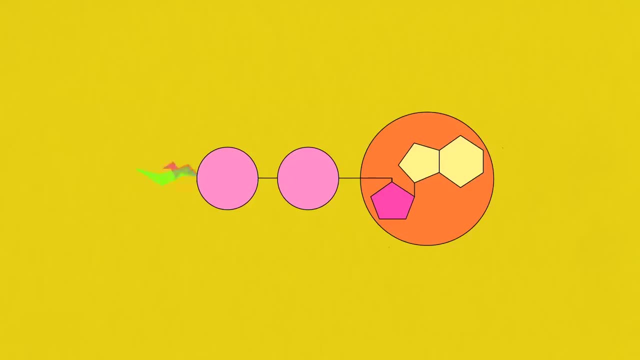 ATP is able to do this nifty trick where it shoots one of the phosphates. This phosphate groups off the end of the seat, creating ADP or adenosine diphosphate, because now there are just two kids sitting on the bus seat. 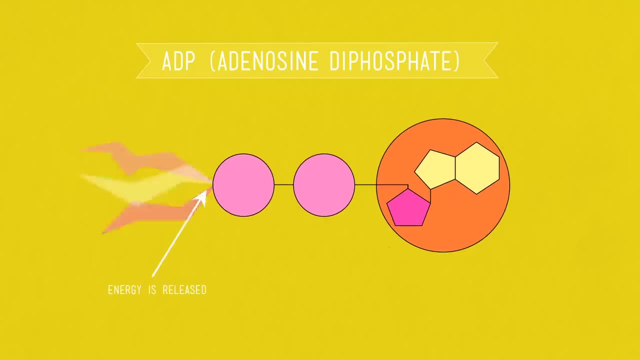 In this reaction, when the third jerk kid is kicked off the seat, energy is released And since there are a lot of water molecules just floating around nearby, an OH pairing that's called a hydroxide from one of the H2Os comes over and takes the place of that third phosphate group. 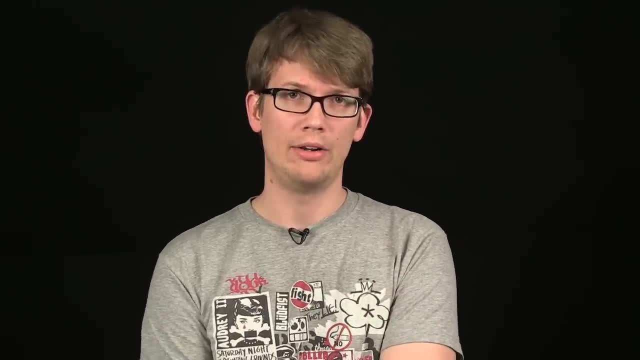 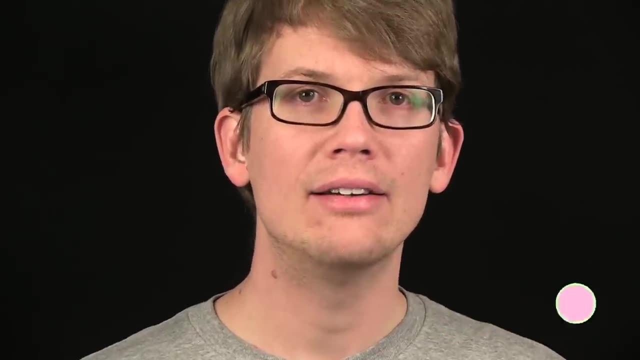 and everybody is much happier. By the way, when you use water to break down a compound like this, it's called hydrolysis- hydro from water and lysis from the Greek word for separate. So now that you know how ATP is spent, let's see how it is minted nice and new by cellular respiration. 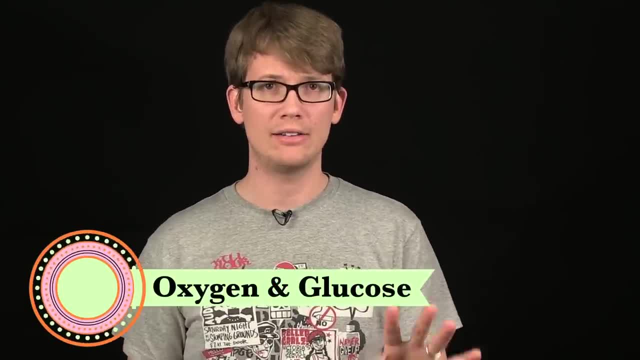 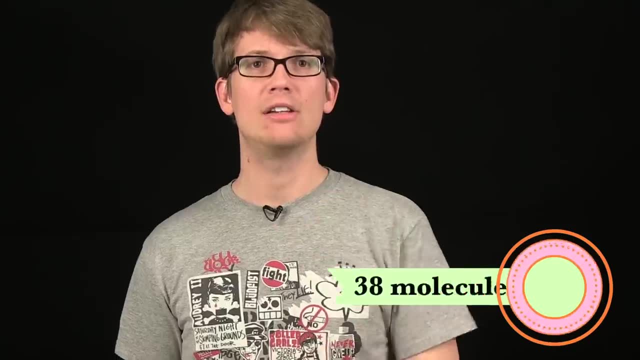 Like I said, it all starts with oxygen and glucose. In fact, textbooks make a point of saying that through cellular respiration, one molecule of glucose can yield a bit of heat and 38 molecules of ATP. Now, it's worth noting that this number is kind of a best-case scenario. 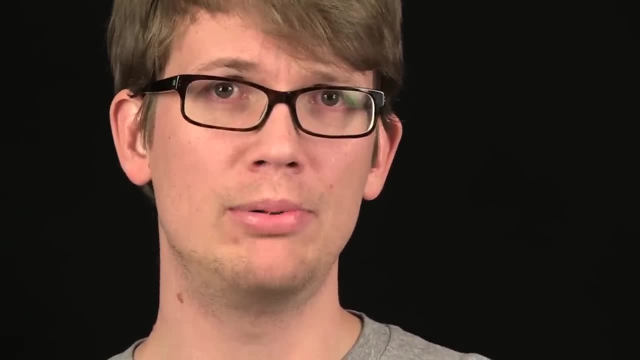 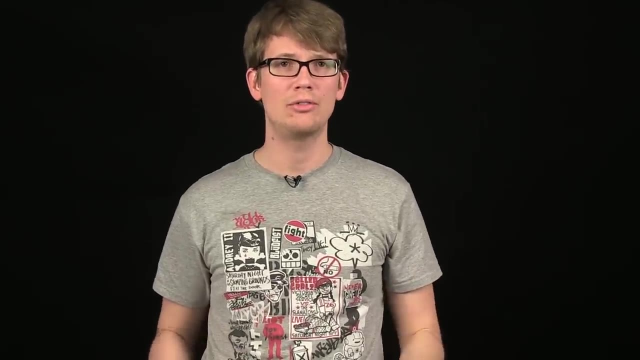 Usually it's more like 29 or 30 ATPs, but whatever, People are still studying this stuff, so let's stick with that number 38.. Cellular respiration isn't something that just happens all at once. Glucose is transformed into ATPs over three separate stages. 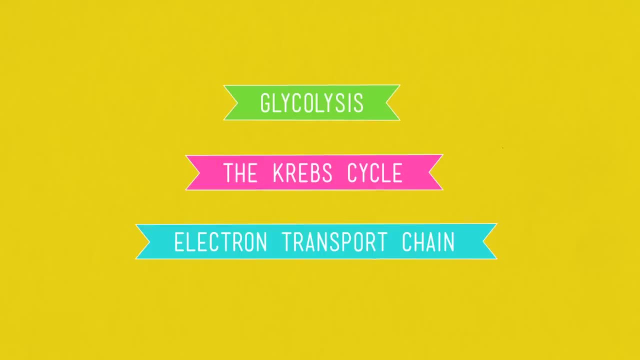 glycolysis, the Krebs cycle and the electron transport chain. Traditionally these stages are described as coming one after the other, but really everything in the cell is kind of happening all at the same time. But let's start with the first step: glycolysis, or the breaking down of the glucose. 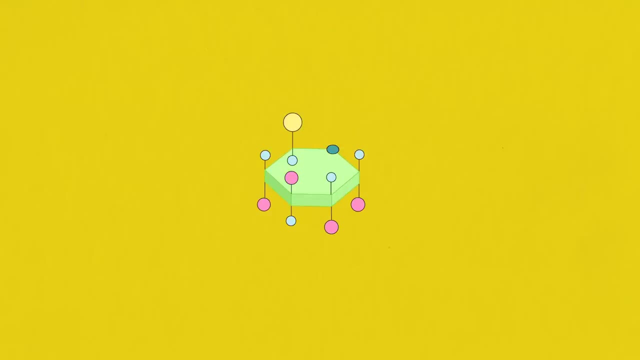 Glucose, of course, is a sugar- You know this because it's got an OSE at the end of it- And glycolysis is just the breaking up of glucose's six-carbon ring into two three-carbon molecules called pyruvic acids or pyruvate molecules. 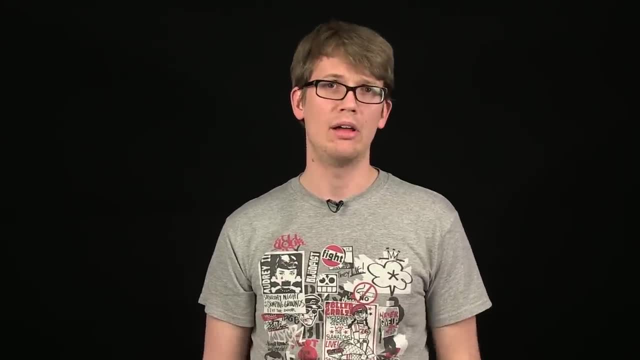 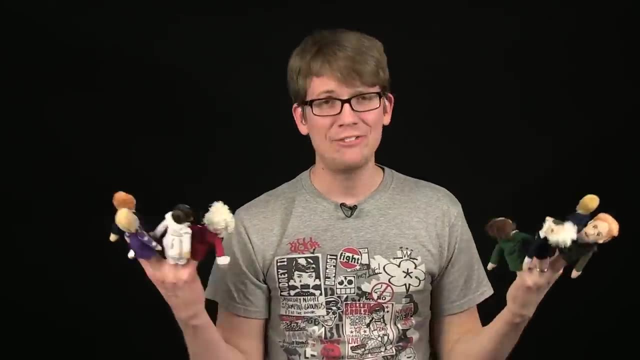 Now, in order to explain exactly how glycolysis works, I'd need about an hour of your time and a giant cast of finger puppets, each playing a different enzyme, And though it would pay me to do it, I would have to use words like phosphoglucoisomerase. 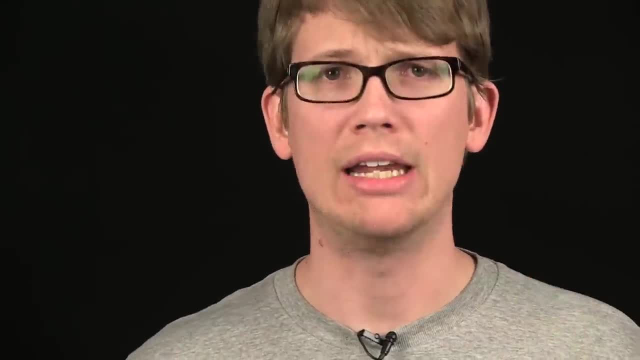 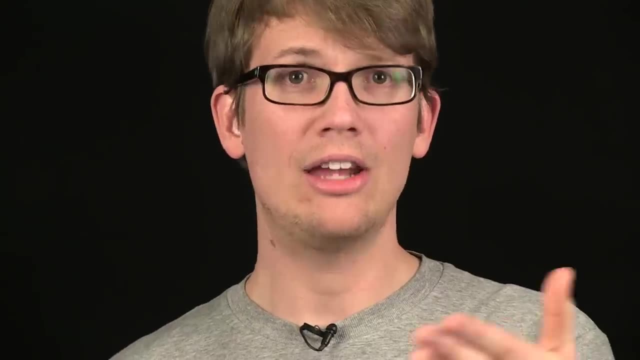 But a simple way of explaining it is like this: If you want to make some money, you gotta spend some money. Glycolysis needs the investment of two ATPs in order to work and in the end, it generates four ATPs, for a net profit, if you will, of two ATPs. 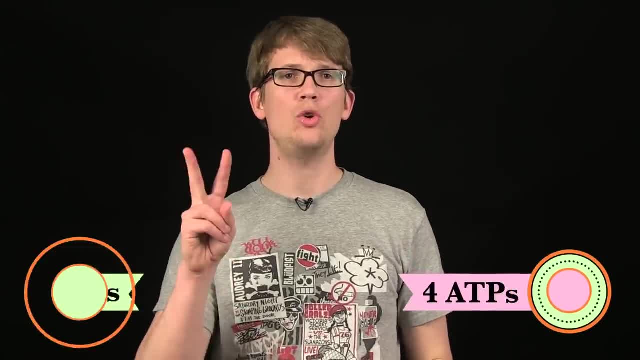 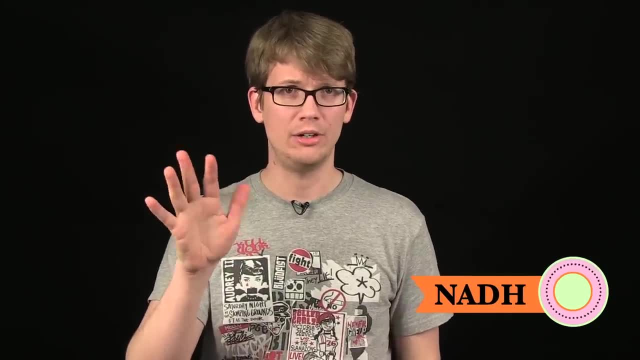 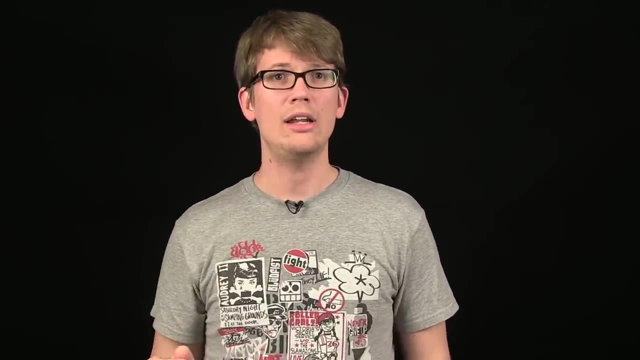 In addition to those four ATPs, glycolysis results in two pyruvates and two super energy-rich morsels called NADH, which are sort of the love children of a B vitamin called NAD+, pairing with energized electrons and a hydrogen to create storehouses of energy that will later be tapped to make ATP. 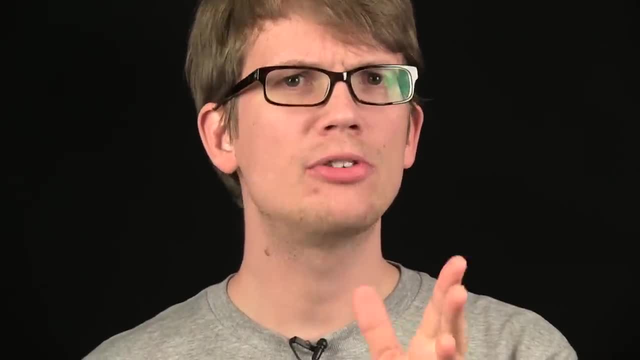 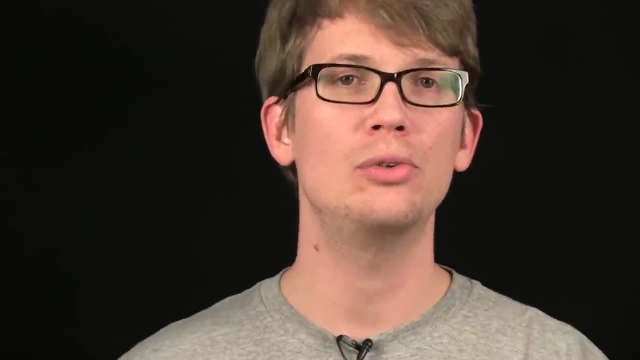 To help us keep track of all the awesome stuff we're making here, let's keep score. So far, we've created two molecules of ATP and two molecules of NADH, which will be used to power more ATP production later. Now a word about oxygen. 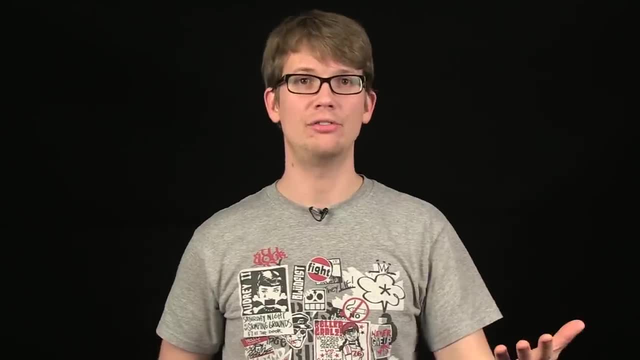 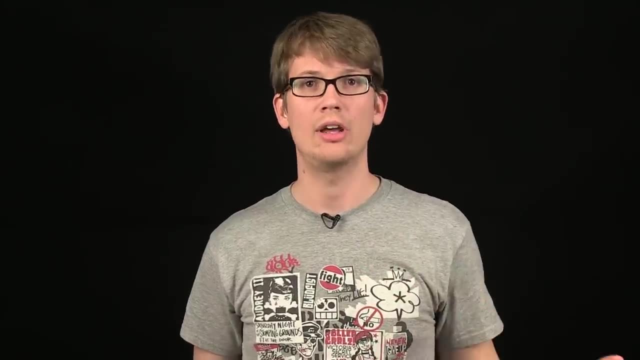 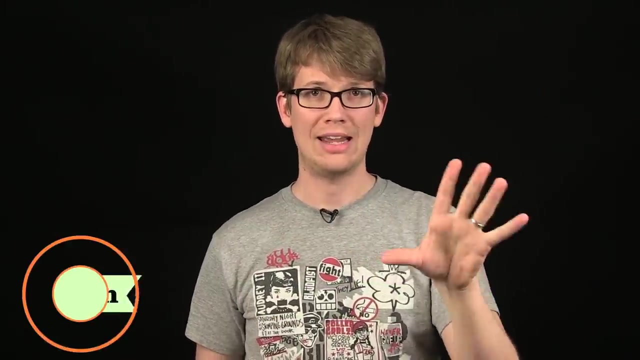 Like I mentioned, oxygen is necessary for the overall process of cellular respiration, but not every stage of it. Glycolysis, for example, can take place without oxygen, which makes it an anaerobic process. In the absence of oxygen, the pyruvates formed through glycolysis gets rerouted into a process called fermentation. 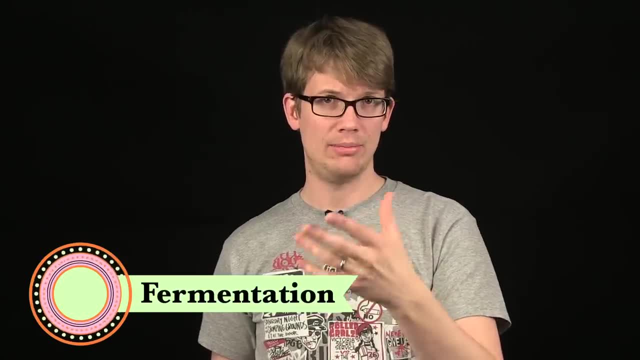 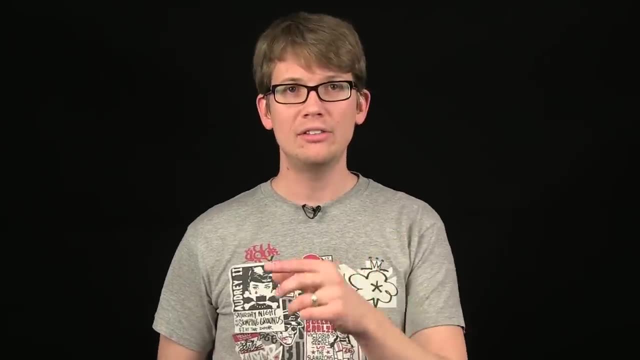 If there's no oxygen in the cell, it needs more of that NADH to keep the glycolysis going. so fermentation frees up some NADH, which happens to create some interesting byproducts. For instance, in some organisms like yeasts the product of fermentation is ethyl alcohol. 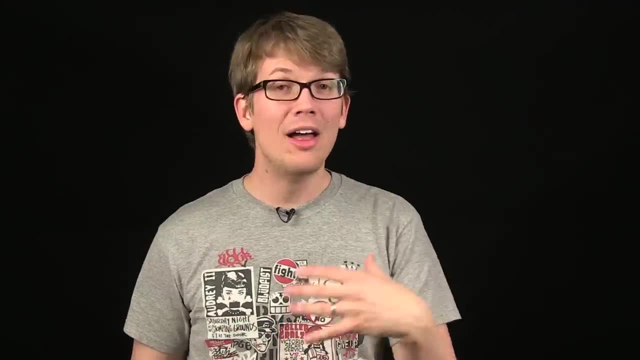 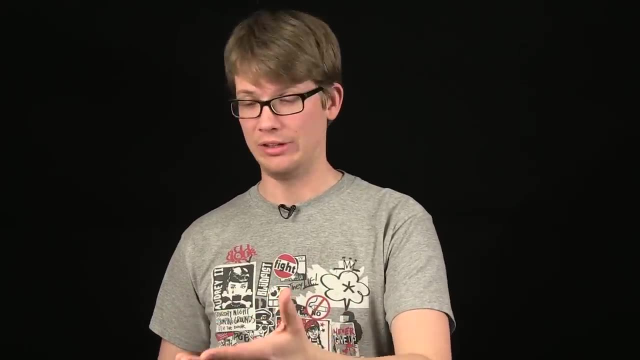 which is the same thing as all of this lovely stuff, But luckily for our day-to-day productivity, our muscles don't make alcohol when they don't get enough oxygen. If that were the case, working out would make us drunk, which actually would be pretty awesome. 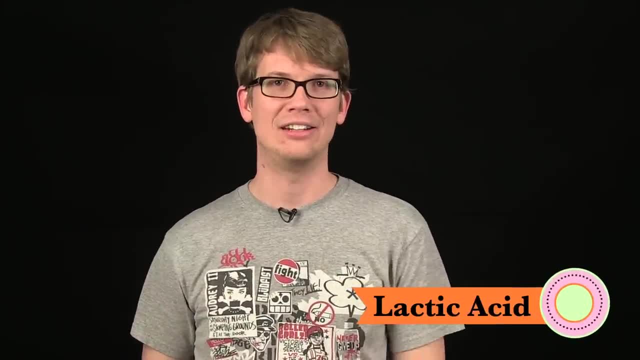 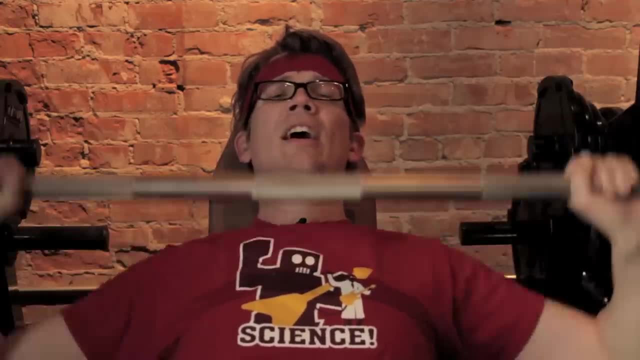 But instead of ethyl alcohol, we need lactic acid, which is what makes you feel sore after that workout that kicked your butt. So your muscles used up all the oxygen they had and they had to kick into anaerobic respiration in order to get the energy that they needed. 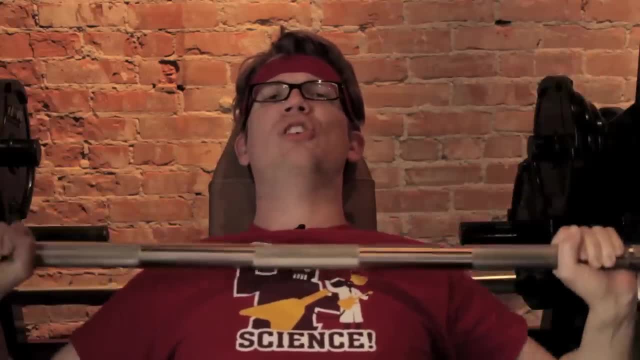 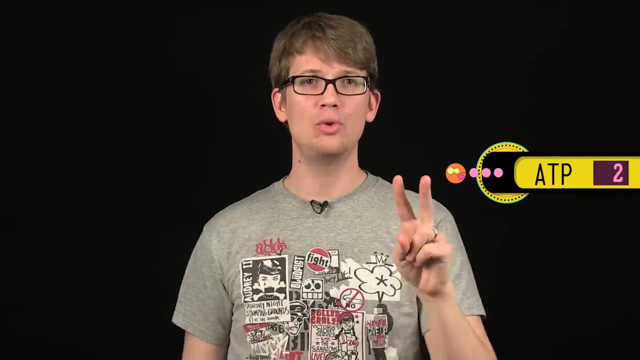 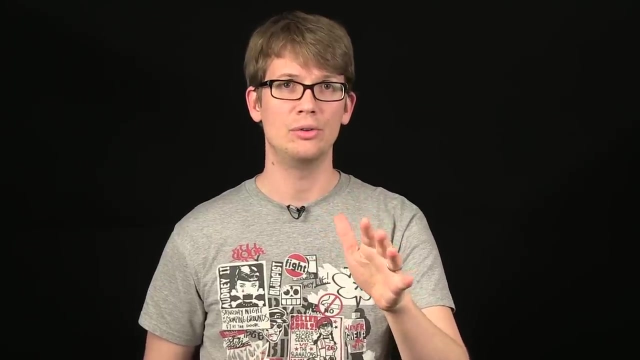 And so you have all this lactic acid building up in your muscle tissues. Ah, Ah, Ah. Back to the score. Now. we have made two molecules of ATP through glycolysis, but your cells really need the oxygen in order to make the other 30-some molecules that they need. 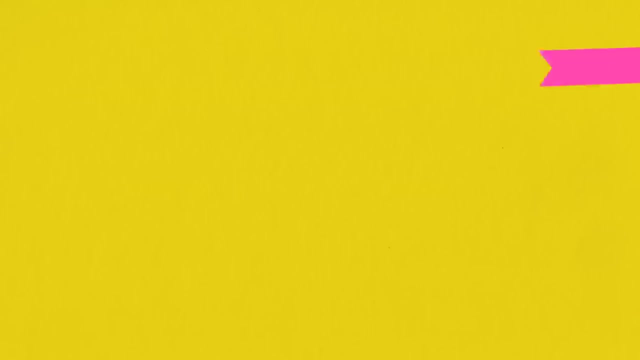 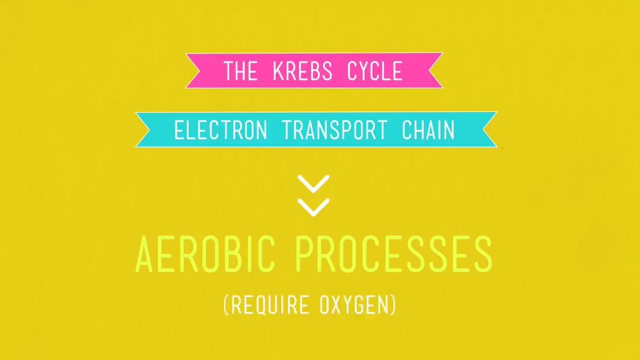 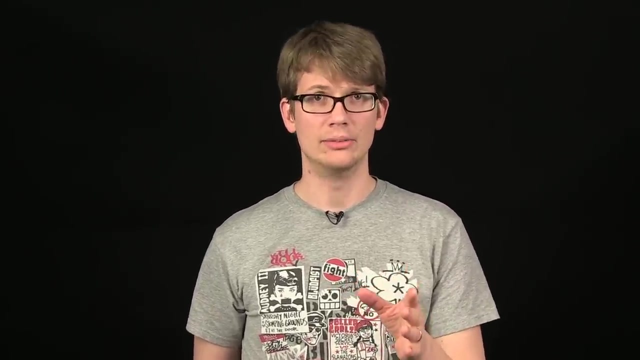 and that is because the next two stages of cellular respiration- the Krebs cycle and the electron transport chain- are both aerobic processes, which means that they require oxygen. And so we find ourselves at the next step in cellular respiration: After glycolysis comes the Krebs cycle. 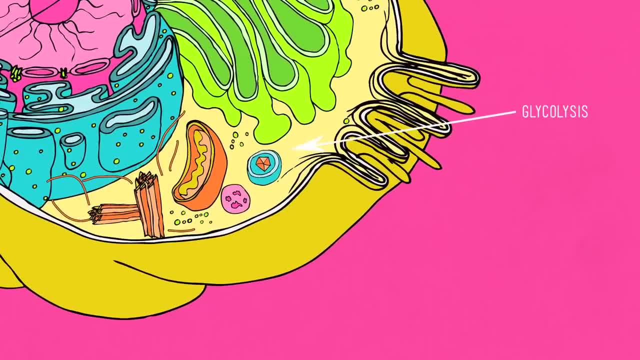 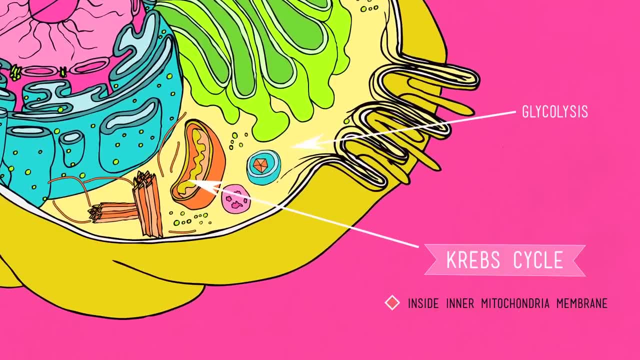 So, while glycolysis occurs in the cytoplasm or the fluid medium within the cell, that all the organelles hang out in, the Krebs cycle happens across the inner membrane of the mitochondria, which are generally considered the power centers. 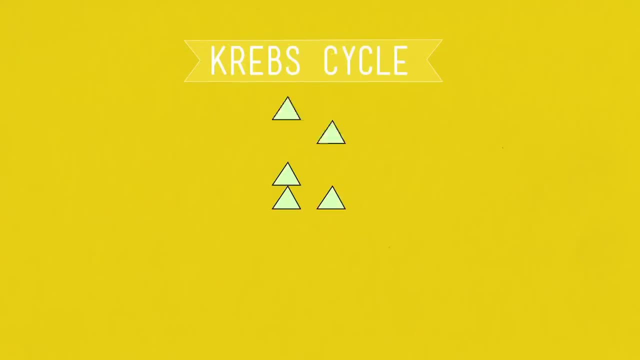 The Krebs cycle takes the products of glycolysis, those carbon-rich pyruvates, and reworks them to create another two ATPs per glucose molecule, plus some energy and a couple of other forms which I'll talk about in a minute. 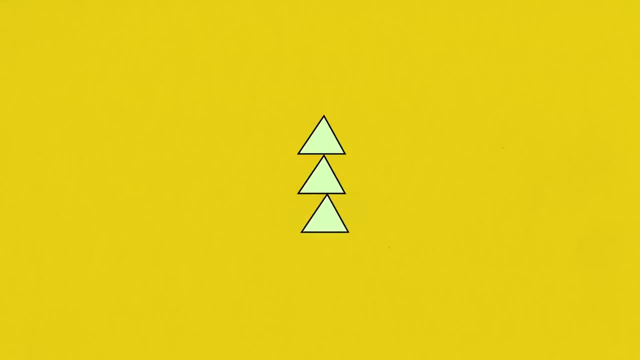 Here's how. First, one of the pyruvates is oxidized, which basically means that it's combined with oxygen. One of the carbons off the three-carbon chain bonds with an oxygen molecule and leaves the cell as CO2.. 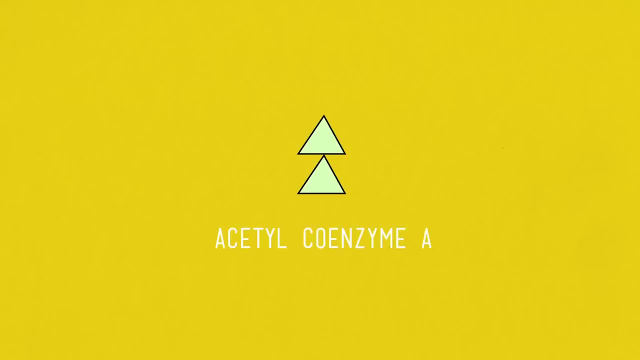 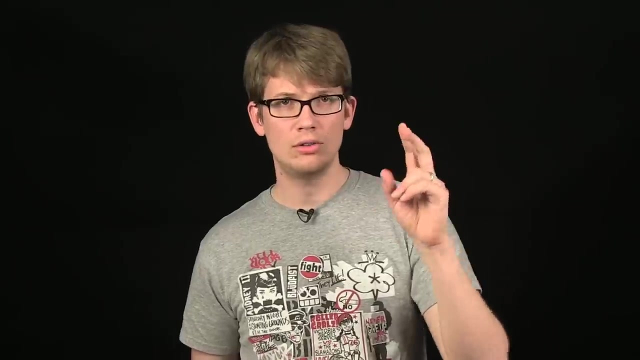 What's left is a two-carbon compound called acetyl coenzyme A or acetyl CoA. Then another NAD plus compound comes along, picks up a hydrogen and becomes NADH. So our two pyruvates create another two molecules of NADH to be used later. 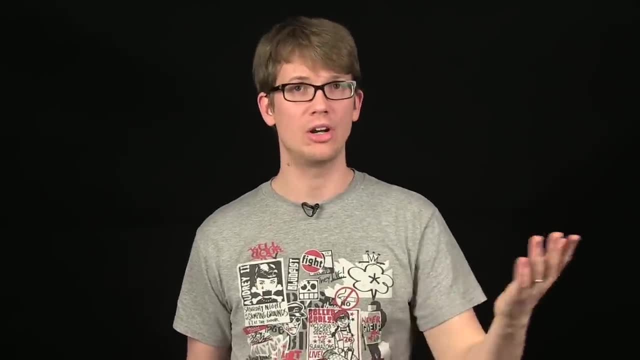 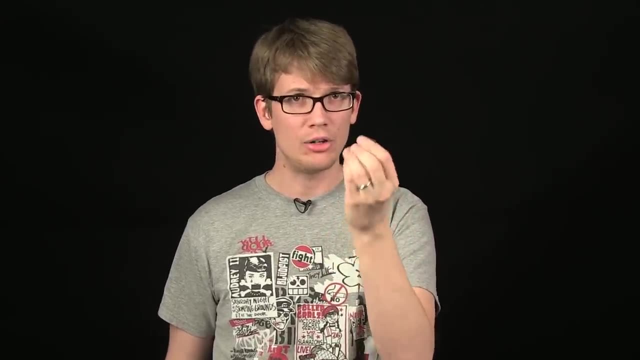 As in glycolysis and really all life, enzymes are essential here. They are the proteins that bring together the stuff that needs to react with each other, and they bring them together in just the right way. These enzymes, for example, bring together a phosphate with an ADP. 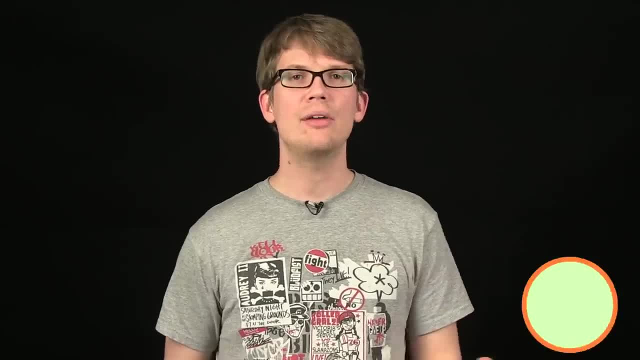 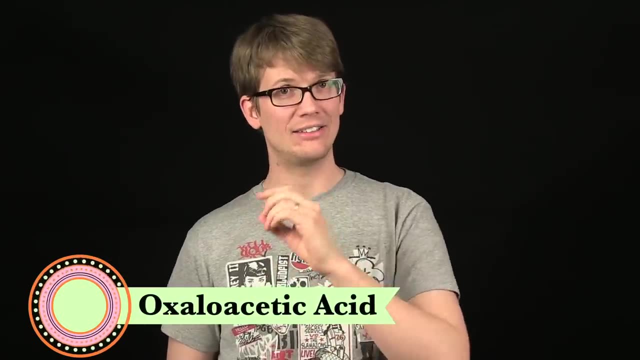 to create another ATP molecule for each. pyruvate Enzymes also help join the acetyl CoA in a four-carbon molecule called oxaloacetic acid- I think that's how you pronounce it together and they form a six-carbon molecule called citric acid. 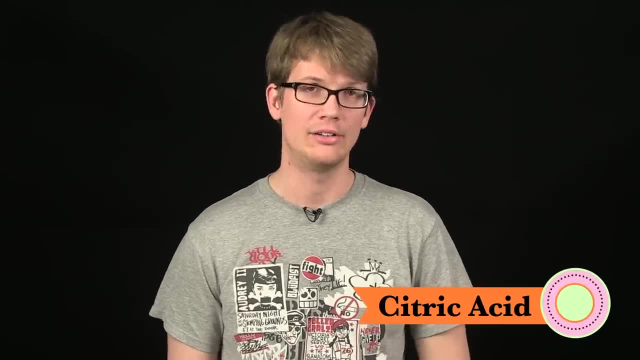 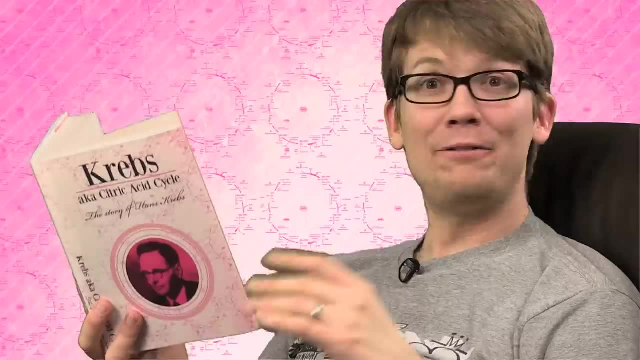 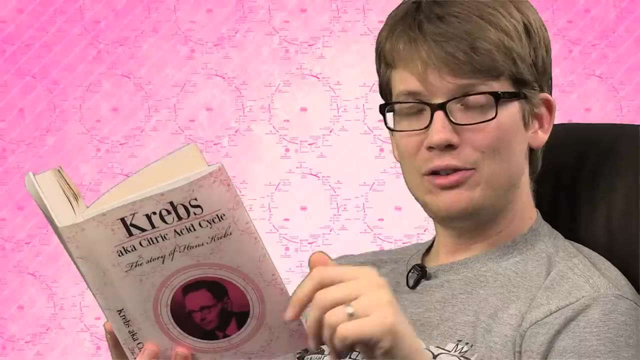 and I'm certain that that's how you pronounce that one, because yeah, it's the stuff that's in orange juice. Fun fact, The Krebs cycle is also known as the citric acid cycle because of this very byproduct. However, it is usually referred to by the name of the man who figured it all out. 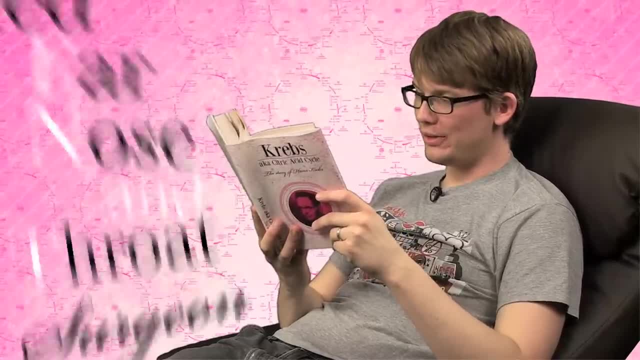 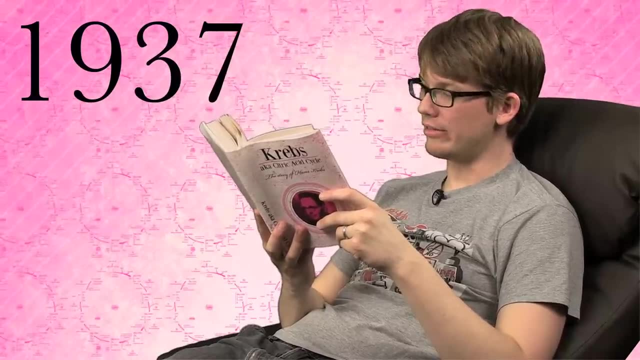 Hans Krebs, an ear, nose and throat surgeon who fled Nazi Germany to teach biochemistry at Cambridge, where he discovered this incredibly complex cycle in 1937.. For being such a total frickin' genius he was awarded the Nobel Prize for Medicine in 1953.. 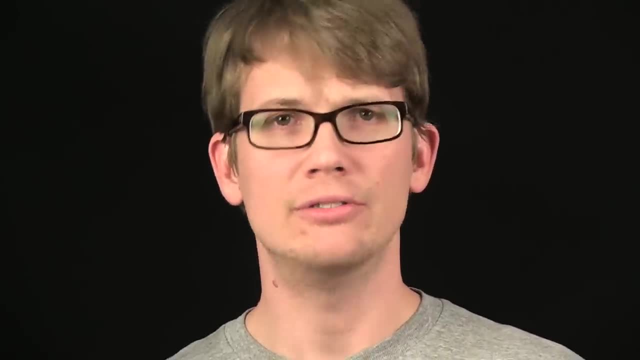 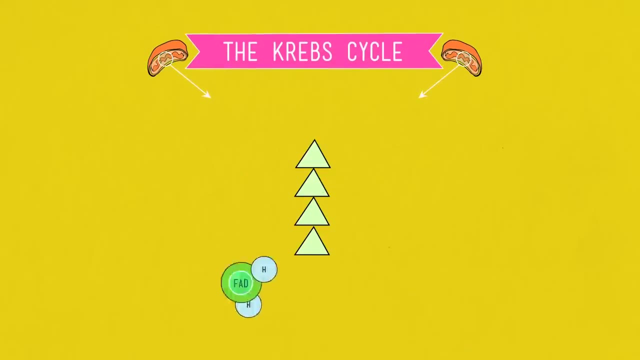 Anyway, the citric acid is then oxidized over a bunch of intricate steps, cutting carbons off left and right, to eventually get back to oxaloacetic acid, which is what makes the Krebs cycle a cycle As the carbons get cleaved off the citric acid. there are leftovers in the form of CO2, or carbon dioxide which are exhaled by the cell and eventually by you, You and I, as we continue our existence as people, are exhaling the products of the Krebs cycle right now. 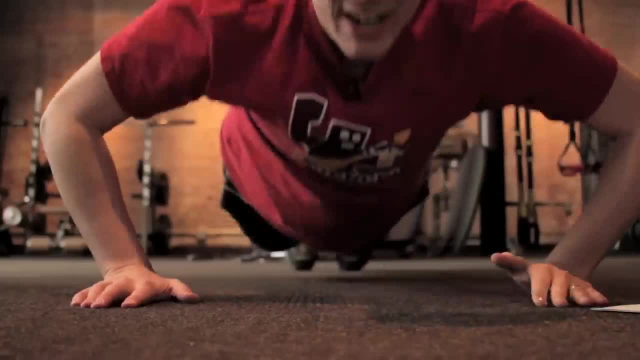 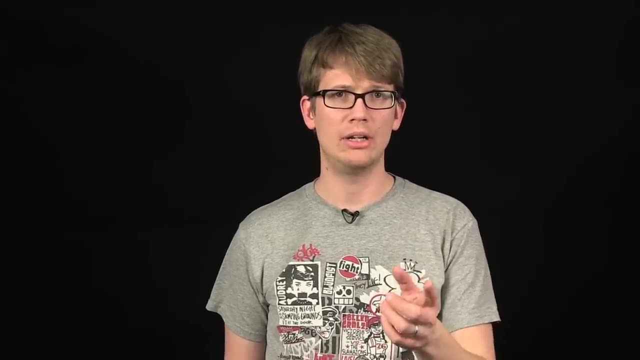 Good work. This video, by the way, using a lot of ATP making it. Now, each time a carbon comes off of the citric acid, some energy is made, but it's not ATP, It's stored in a whole different kind of molecular package. 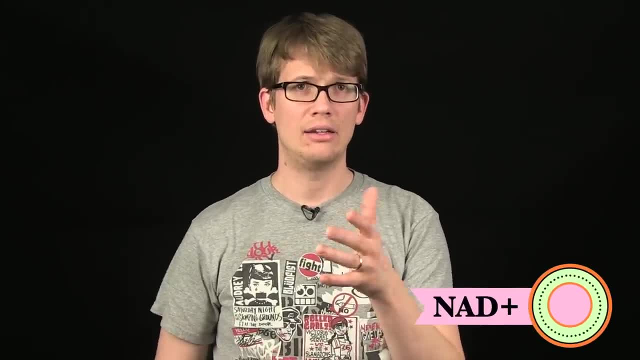 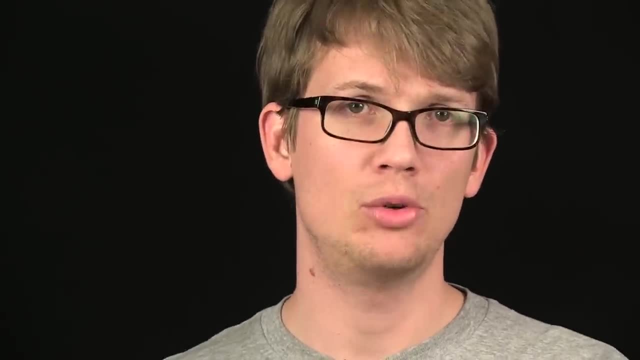 This is where we go back to NAD+ and its sort of colleague, FAD. NAD+ and FAD are chummy little enzymes that are related to B vitamins, derivatives of niacin and riboflavin, which you might have seen in the vitamin aisle. 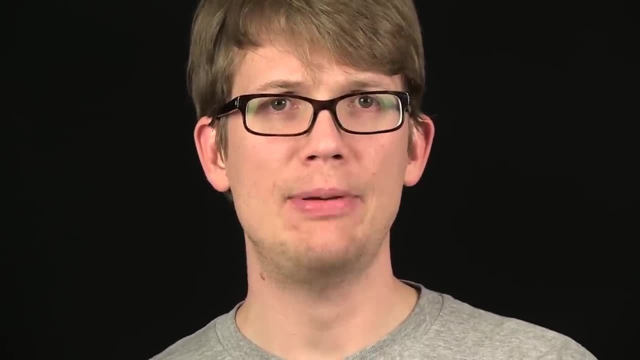 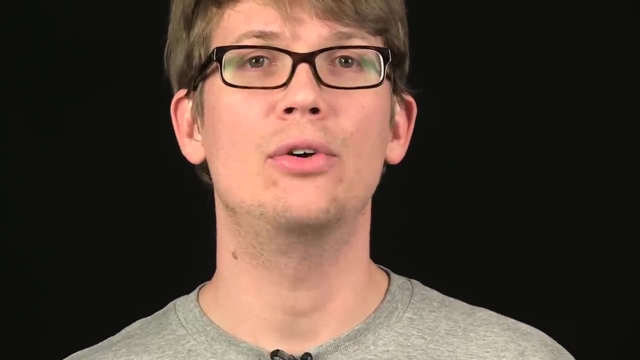 These B vitamins are good at holding on to high energy electrons and keeping that energy until it can get released later in the electron transport chain. In fact, they're so good at it that they show up in a lot in those high energy vitamin powders that the kids are taking these days. 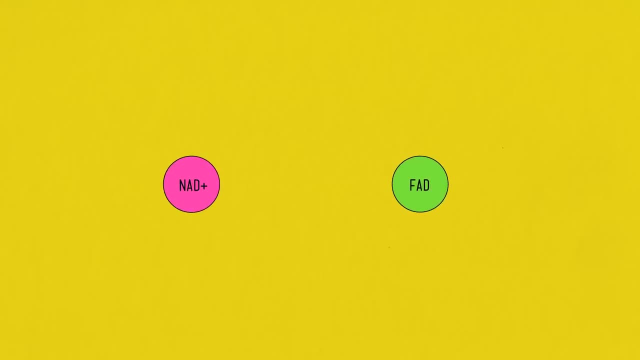 NADs and FADs are like batteries, Big, awkward batteries that pick up hydrogen and energized electrons from each pyruvate, which in effect charges them up. The addition of hydrogen turns them into NADH and FADH2, respectively. 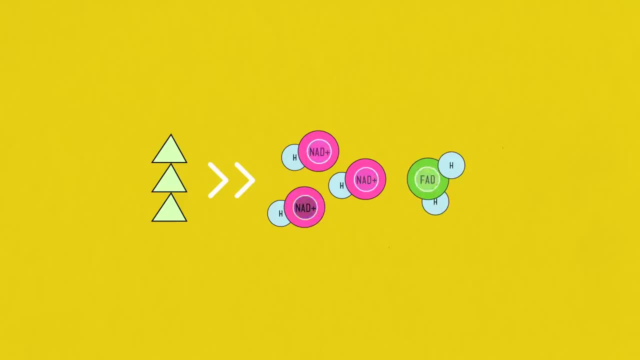 Each pyruvate yields three NADHs and one FADH2 per cycle And since each glucose has been broken down into two pyruvates, that means that each glucose molecule can produce NADHs and two FADH2s. 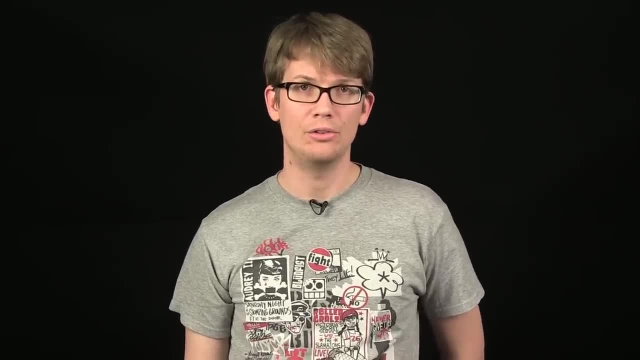 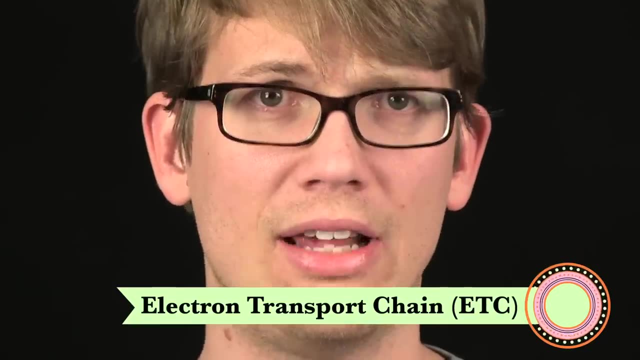 The main purpose of the Krebs cycle is to make these powerhouses for the next and final step, the electron transport chain. Now comes the time when you're saying Sweet pyruvate sandwiches, Hank. Aren't we supposed to be making ATP here? 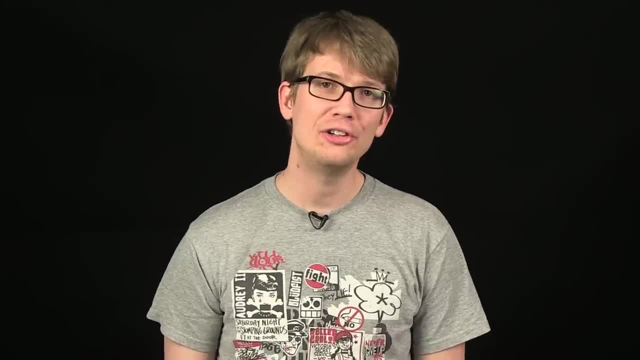 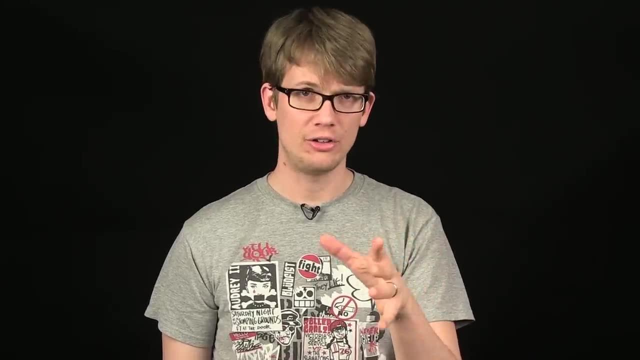 Let's make it happen, Cap'n. What's the holdup? Well, friends, your patience is finally paying off, because, when it comes to ATPs, the electron transport chain is the real moneymaker. In a very efficient cell, it can net a whopping 34 ATPs. 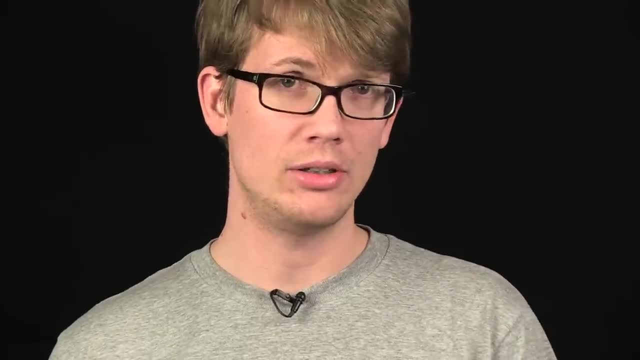 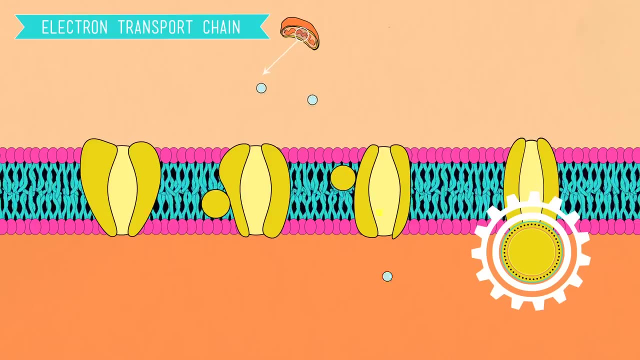 Remember all those NADHs and FADH2s that we made in the Krebs cycle. Well, their electrons are going to provide the energy that will work as a pump along a chain of channel proteins across the inner membrane of the mitochondria where the Krebs cycle occurred. 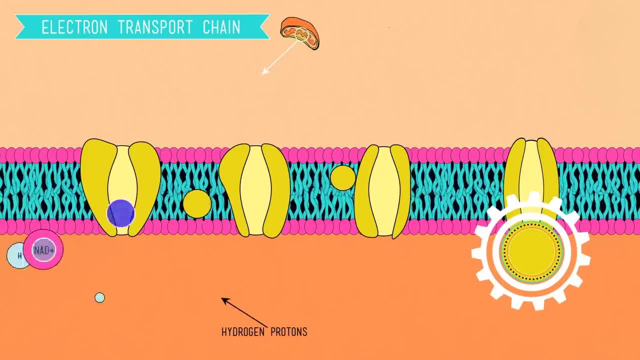 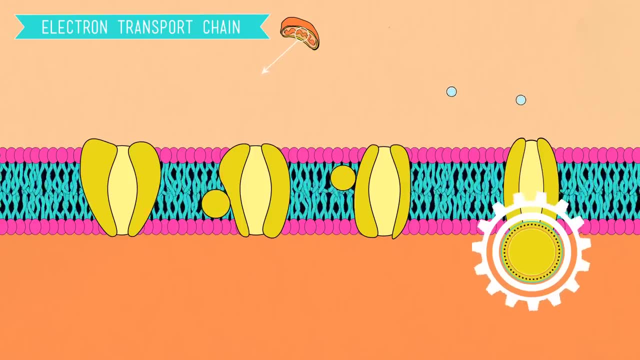 These proteins will swap these electrons to send hydrogen protons from inside the very center of the mitochondria across its inner membrane to the outer compartment of the mitochondria. But once they're out, the protons want to get back to the other side of the inner membrane. 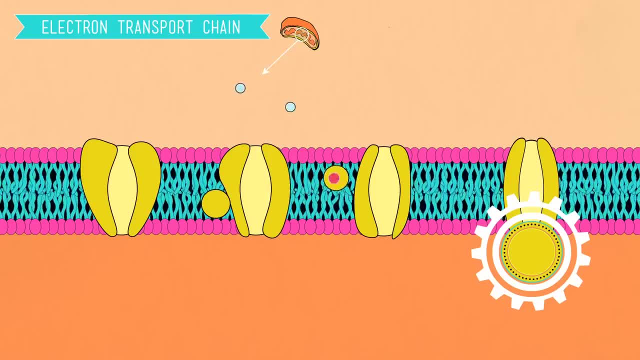 because there's a lot of other protons out there And, as we've learned, nature always tends to seek a nice, peaceful balance on either side of a membrane. So all these anxious protons are allowed back in through a special protein called ATP synthase. 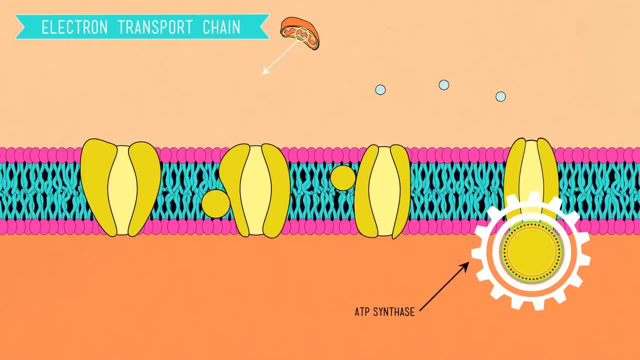 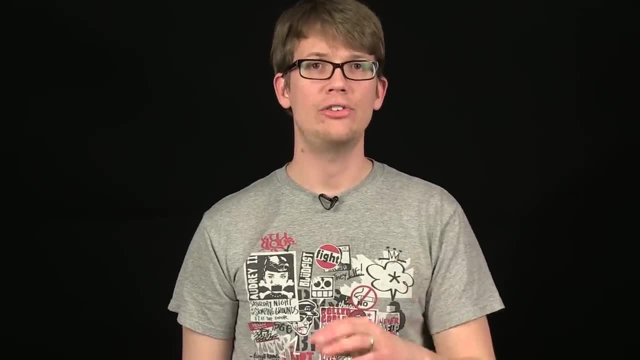 And the energy of this proton flow drives this crazy spinning mechanism that squeezes some ADP and some phosphates together to form ATP. So the electrons from the 10 NADHs that come out of the Krebs cycle have just enough energy to produce roughly 3 ATPs each.